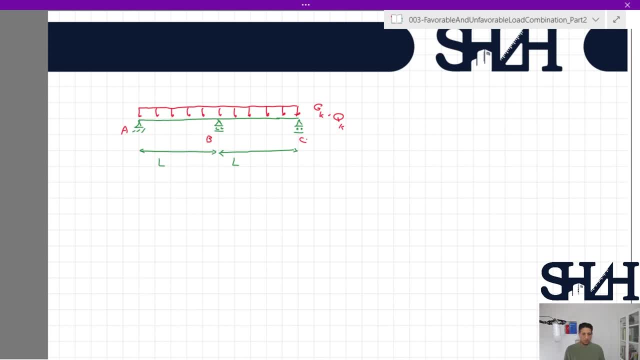 moment is not in the center of the beam. If the load is distributed in two spans, the maximum bending moment is in the center of A and B supports And we'll see it will be in the 3 over 8 of L from point A and the same from point C. But when it comes to the worst live load appearance, assuming that the permanent action is not critical to be considered for superior and inferior, then we have only one GK which can be in the superior as unfavorable and also inferior for the most favorable action. 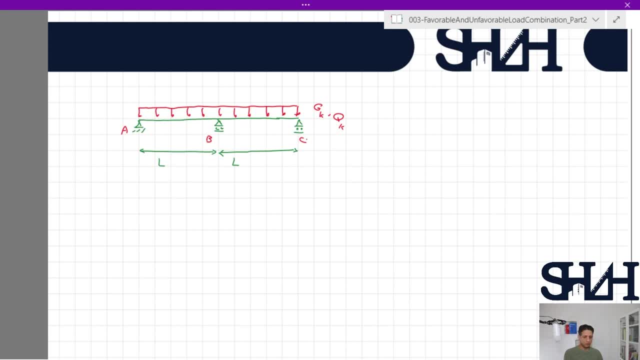 case. But when it comes to the live load, the effect of live load being in two spans would affect the maximum bending moment in one span. For analyzing this beam you can use different methods. for example, force method can be one, slope deflection or any other kind might be appropriate. So what we can do for the entire load applied to the 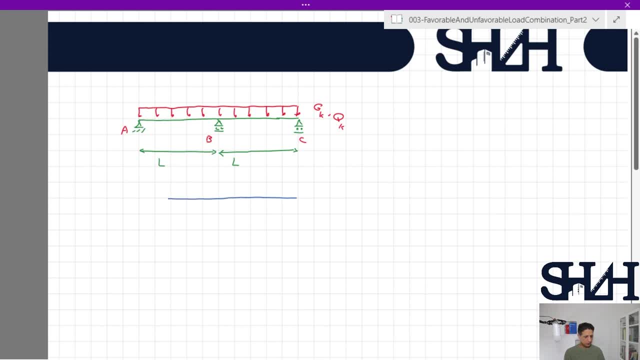 section, I use superposition method. I'll sketch one beam, A, C and this is point B- under Q plus the other beam with the reaction force of RB. Based on the tables that you can find easily here and there, the deflection in the center of a beam under distributed load of Q will be 5 Q L power by 4 divided by 3 over L. 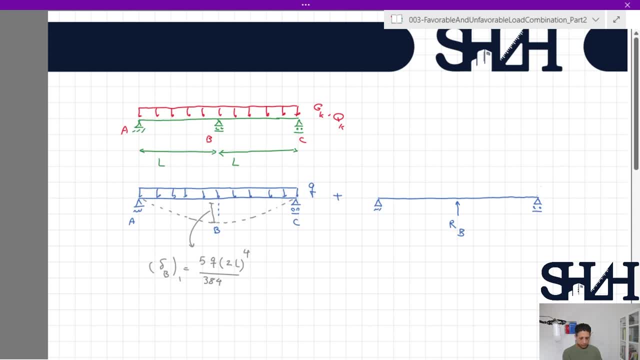 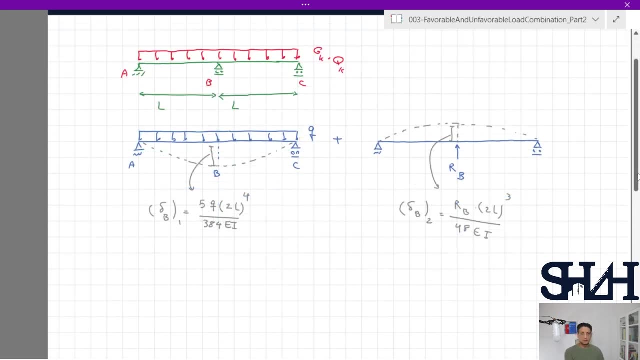 And for a beam with the length of 2 L with the point load in the center. this deflection will be force times length. power by 3 divided by 48 EI, This one as well. As far as in the main beam, the deformation at point B is 0, meaning that delta B1 downward should be the same as delta B2 upward. As a result, 5 Q L. power by 3 over L. 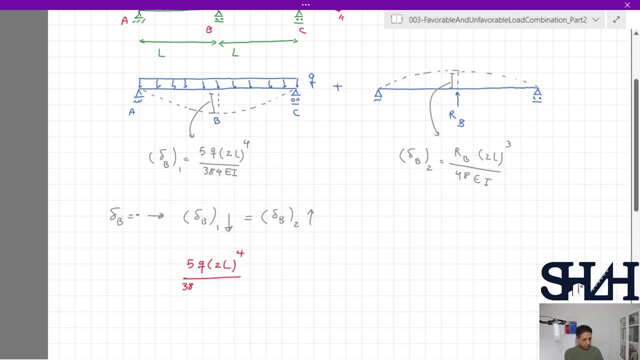 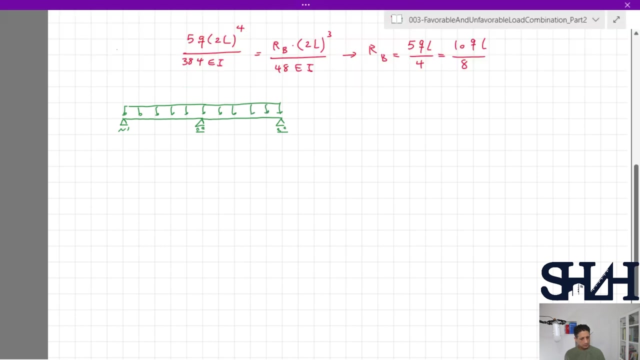 Q 2 L power by 4 divided by 384 EI equals to RB times 2 L power by 3 divided by 48 EI. As a result, reaction at point B will be 5 Q L over 4 or 10 Q L divided by 8.. If you have the support reaction in the center, then easily we can find out the other reactions as far as it's completely symmetrical. So this will be: 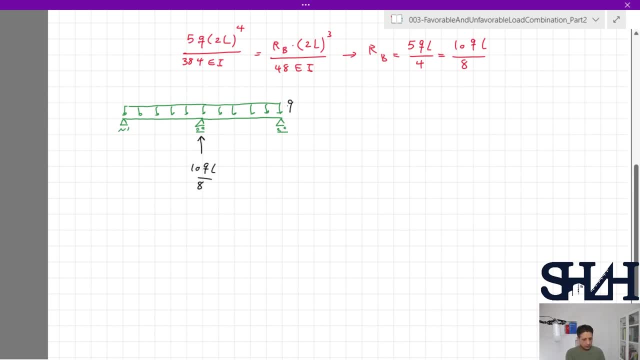 10 Q L divided by 8, and this is Q, the total value of the force. So EI and CY are the same. EI equals to CY and it will be Q times 2 L minus 10 Q L divided by 8, divided by 2.. 3 Q L divided by 8.. And then we can sketch here force and bending moment for this beam. As I said, you can use any other methods. 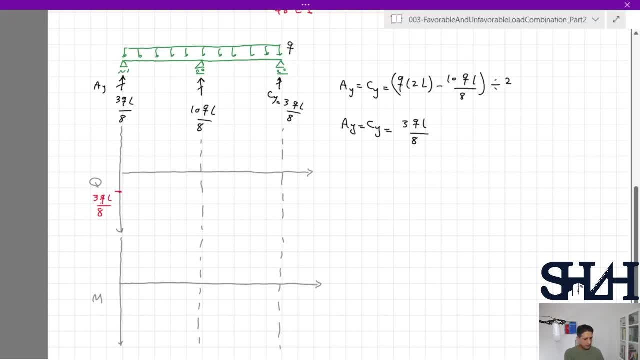 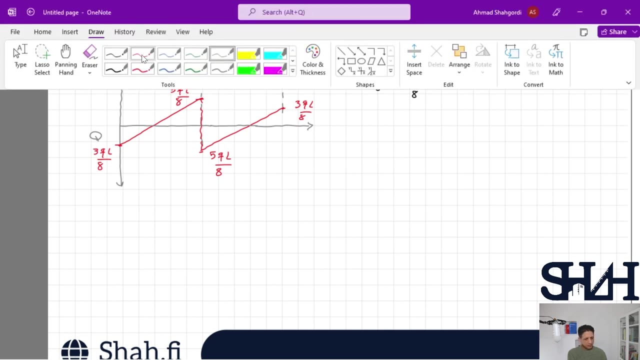 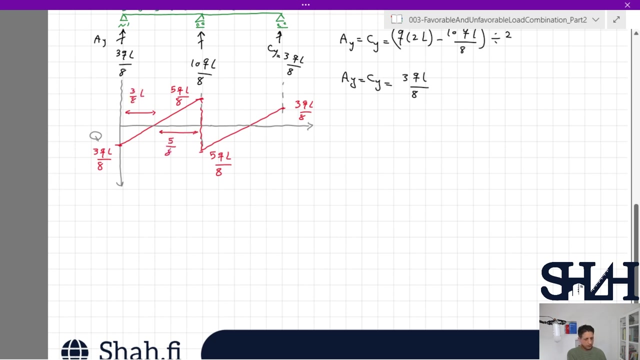 For this calculation: 3 Q L over 8, and then it comes to 5 Q L over 8.. Now to sketch the bending moment diagram, we just need to calculate the area of shear force or shear diagram. This is 3 over 8 L and the rest 5 over 8 L. The area for the first part will be 9 over 128. 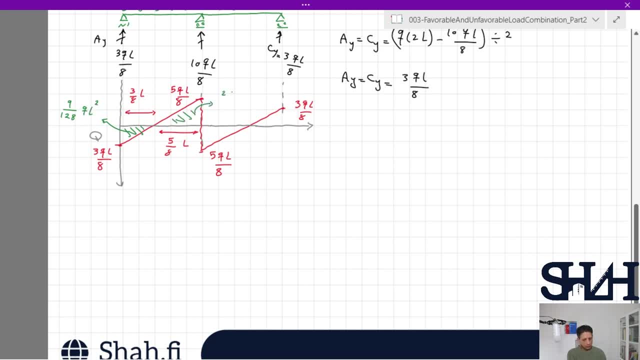 8 Q L square, and here it will be 25 divided by 128 Q L square, The same value for the other sides. And now we can sketch the bending moment diagram. In the beginning the bending moment is 0.. It comes to 9 over 128 Q L square, and then minus 25 will be minus 16 Q L square divided by 128, which is Q L square divided by 8.. 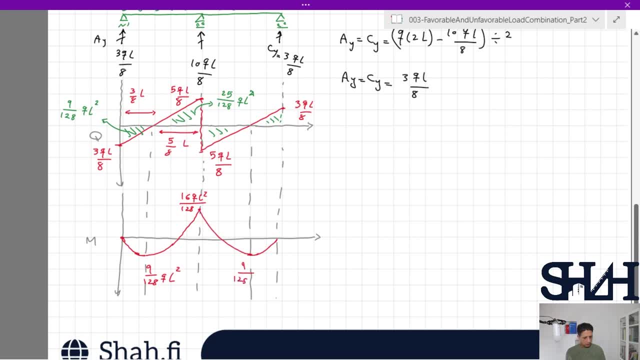 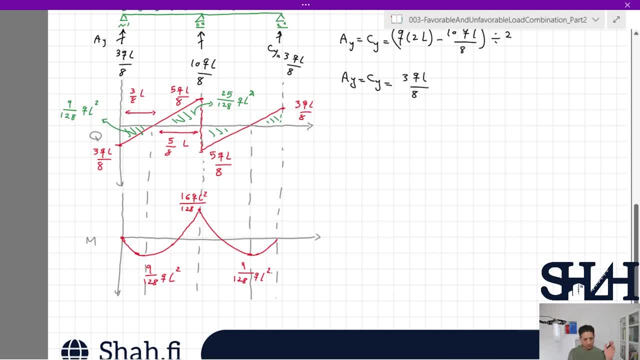 which is not in the center. it is in the distance of 3 over 8 L. so this can be used for a permanent action when the structure is not sensitive to the permanent load. but when it comes to live load, the position of light load would affect the maximum bending moment. if it is coming in two spans, then 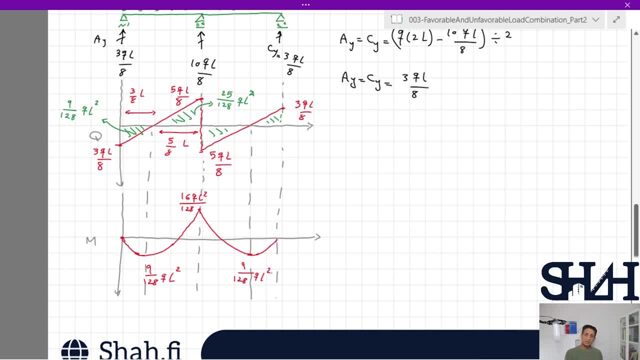 it is favorable because it is reducing the maximum bending moment. as a result, when we are interested in finding out the maximum bending moment, especially for live load, the position of live load is very important if, especially if the structure is complicated for many structures, when the beams are. 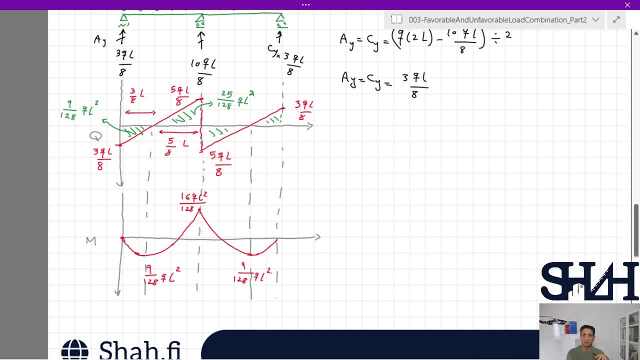 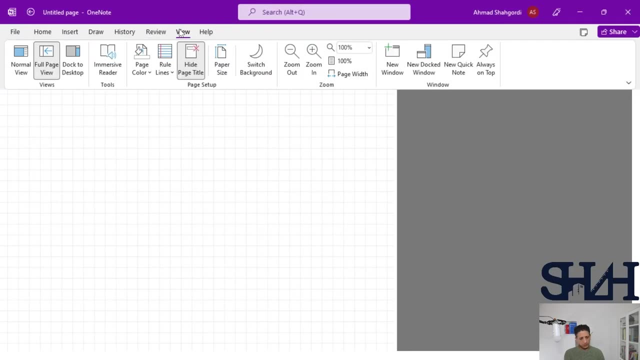 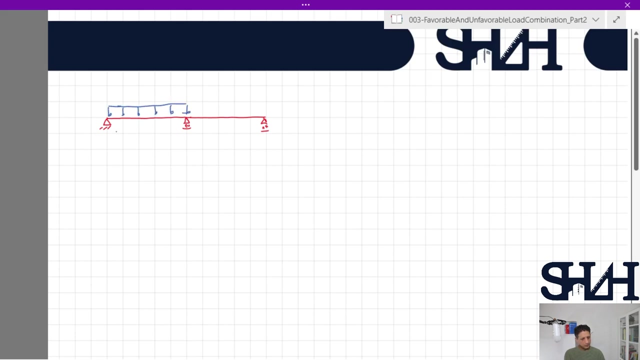 really supported on columns on core wells. perhaps this is not relevant, but when it comes to complicated structures then this is very important uh factor for finding the maximum bending moment. now we can go to applying the load only on one span. assume that the load is applied only on one span here, a span AB, and the other one is without any uh load. so for analyzing, 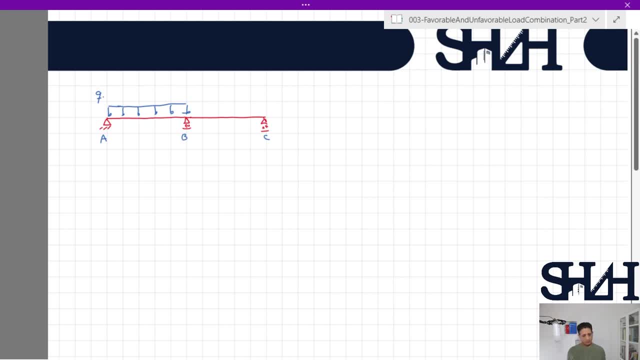 this beam we can use different methods, for example slope deflection or other methods. here I'm going to use the combination of uh direct and indirect symmetric principle. so every structure, if they are symmetric based on their appearance, regardless of the load, can be written as the summation of two. 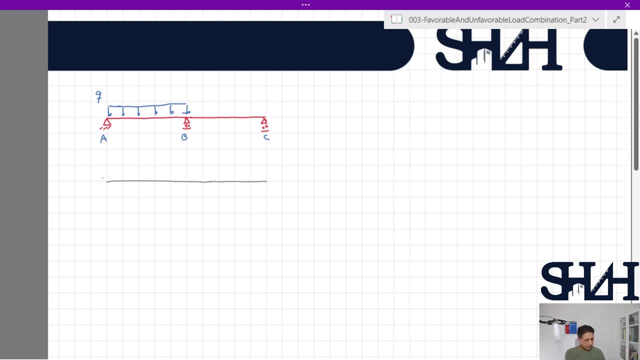 different beams. for example, here I can write it down: this is one beam with the load of q divided by two, plus the same beam q divided by two on one span and minus q divided by two on the other side. if you use superposition, you can see that a, b 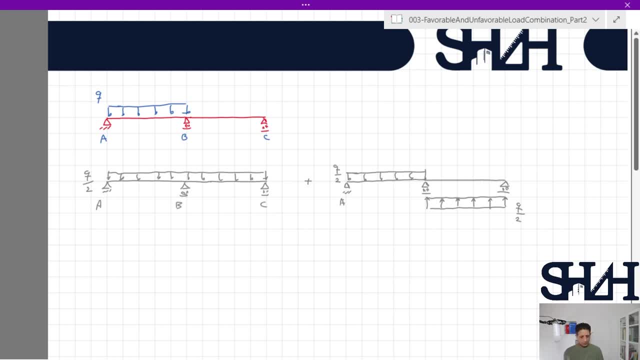 in total will be under q and b. c will be under zero load. they are balancing each other. for the first one, we have the solution already for bending moment from the previous calculation, except the load is half, so it will be in the distance of three over eight l, and this value was 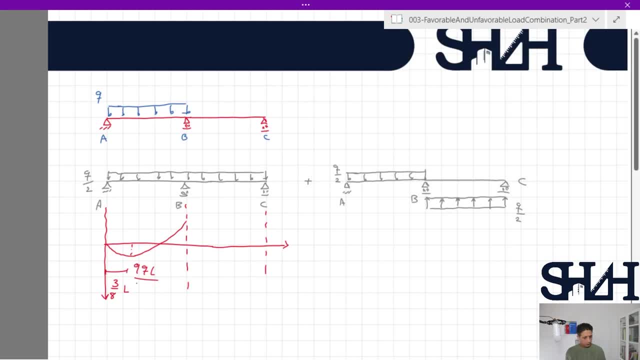 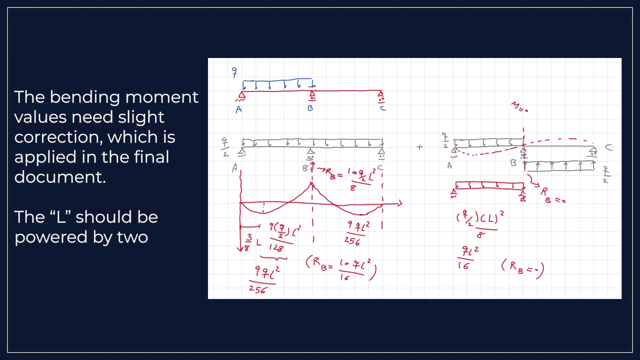 nine q, l divided by 128, which here will be 256 because it is q over two. i can write it down this way: nine q divided by two, l divided by 128. So this will be 9QL divided by 256.. The same happens to the other half, 9QL divided by 256. 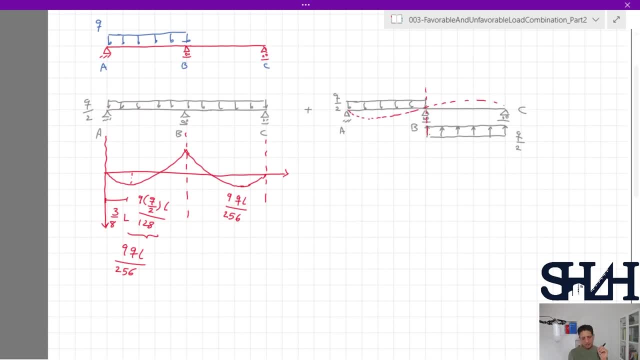 For the other structure, the deformation will be this way: This structure is called reverse symmetric, meaning that the structure itself is symmetric and the loading on the structure is in the opposite direction. So if you have such a situation, then in the center of symmetrical point, bending moment. 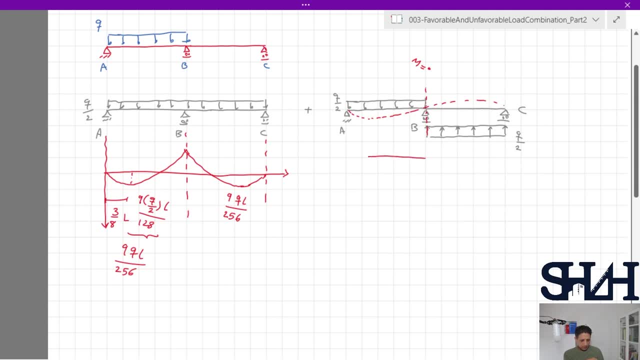 will be zero. As a result, you can easily find out that the system is a simple beam, which the maximum bending moment will be QL squared divided by 8, which is QL squared divided by 16.. And it will happen in the center. 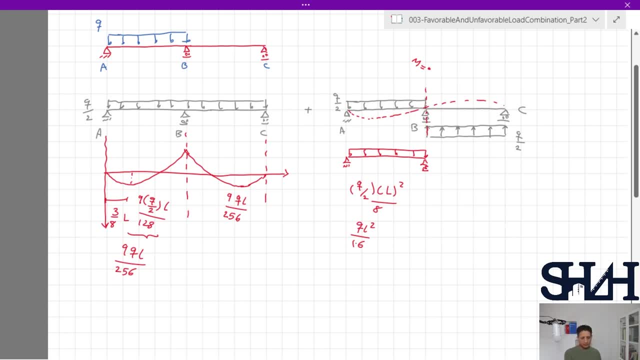 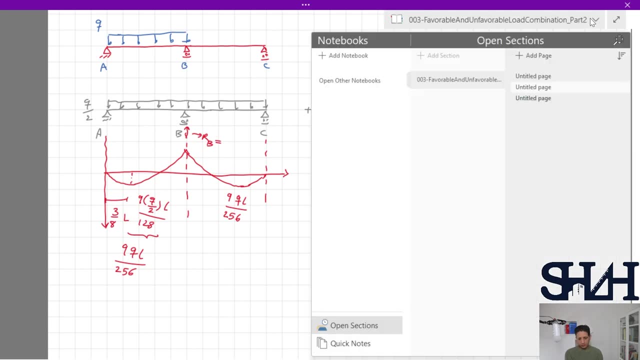 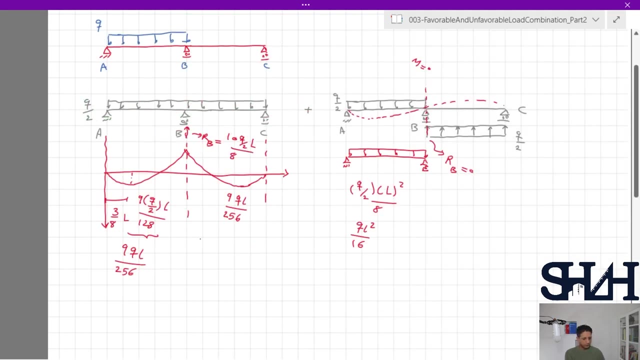 Also, the reaction force at point B in this case will be zero, And here RB was based on our calculation earlier: 10QL over 8, 10UL over 8.. So it will be 0.. This will be RB in this case will be 10QL divided by 16, and RB here will be 0.. 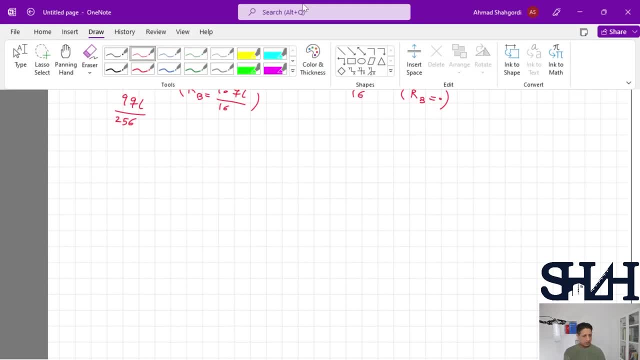 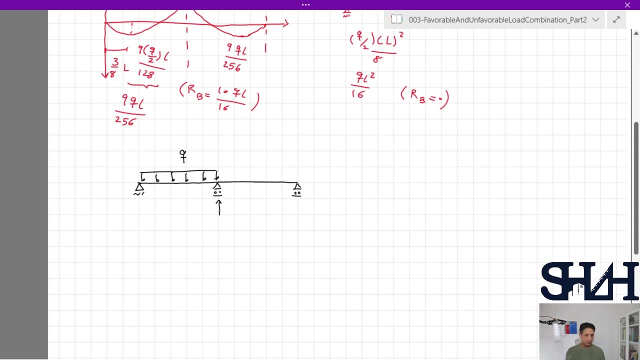 And now, if you sum these two together, you will have the support reaction. at point B, You have load only on one span. So this will be 10QL divided by 16 plus 0.. So it will be 5QL divided by 8.. 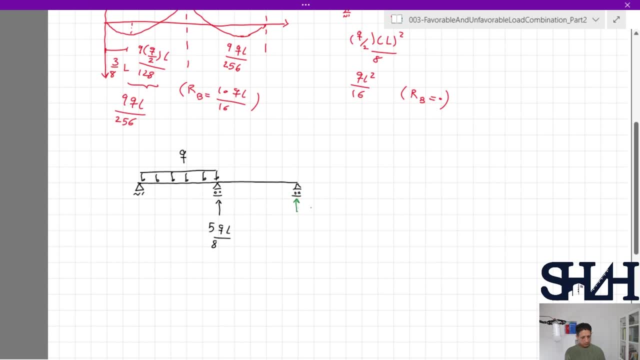 And now you can simply take the moment and find out CY and AY. So this will be 10QL divided by 16 plus 0.. And now you can simply take the moment and find out CY and AY. Sigma M about A equals 0.. QL times L divided by 2 minus 5QL. divided by 8 times L minus CY times 2L equals 0.. Sigma M about A equals 0.. QL times L divided by 2 minus 5QL. divided by 8 times L minus CY times 2L, equals 0.. Sigma M about A equals 0.. QL times L divided by 2 minus 5QL divided by 8 times L minus CY times 2L equals 0.. CY will be 1 over 2 minus 5 over 8 times QL divided by 2.. QL times L divided by 2, minus 5QL divided by 8 times L, minus CY times 2L, equals 0.. CY will be 1 over 2 minus 5 over 8 times QL divided by 2.. So it will be minus QL divided by 16.. 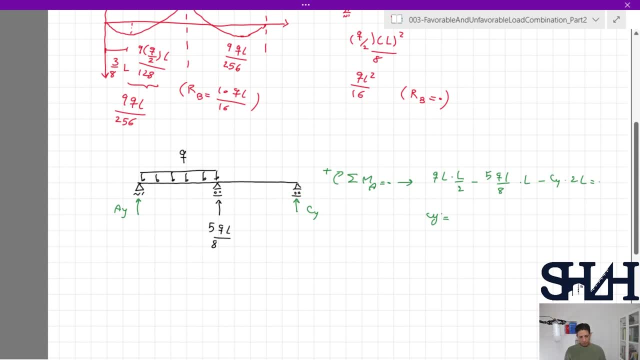 So this value will be UL divided by 16.. So this value will be UL divided by 16.. will be 1 over 2 minus 5 over 8 times ql divided by 2, so it will be minus ql divided by 16.. 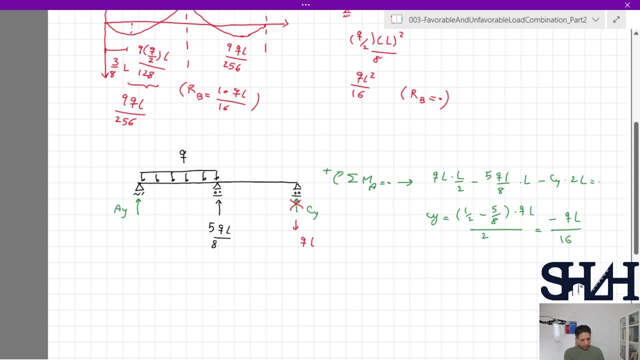 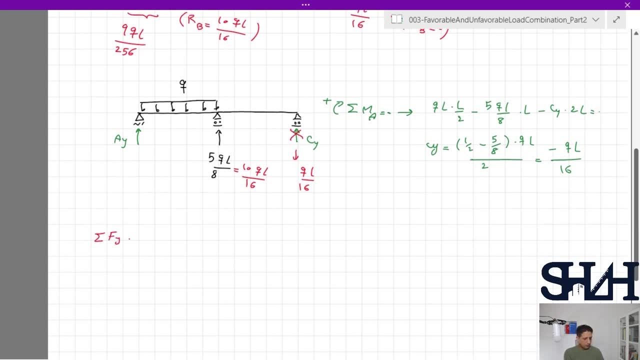 so this value will be ul divided by 16. i prefer to write this down as 10 ql over 16. now sigma fy equals 0, ay minus ql plus 10. ql divided by 16 minus ql divided by 16 equals 0. as a result, ay. 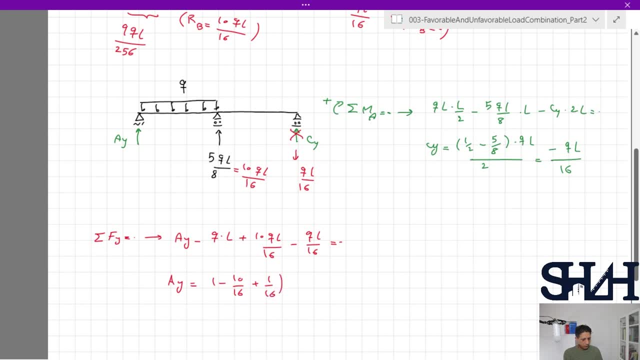 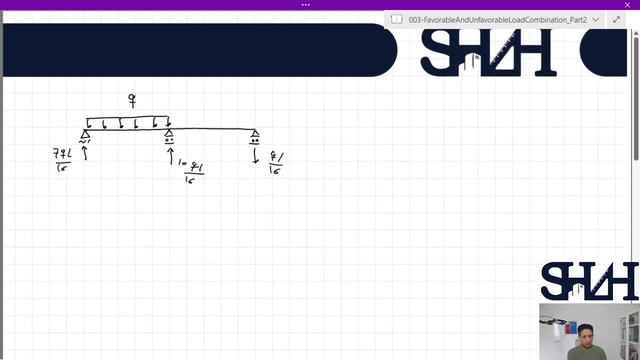 will be 1 minus 10 over 16 plus 1 over 16 times ql. 16 minus 10, 7 ql divided by 16.. and now we have the support reactions. we can sketch the shear force and bending moment there. now we can sketch the 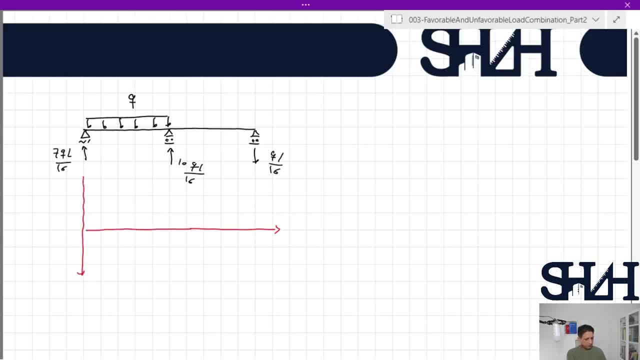 shear force and bending moment for this half loaded beam: 7 ql divided by 16, and then 1 ql is reduced. so here it will be 9 ql divided by 16, and then it will be plus 10, which is 1 ql divided by 16, and finally it will be 0.. 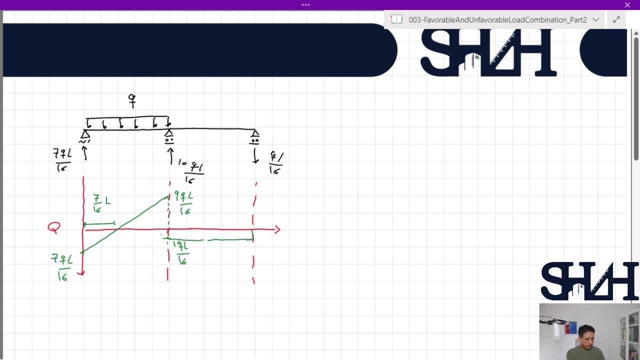 this length will be 7 divided by 16 l, and the other one will be 9 divided by 16 l. now we need to calculate the area of each part. so here it will be 49 q l square divided by 512. the other part will be 81 ql square. 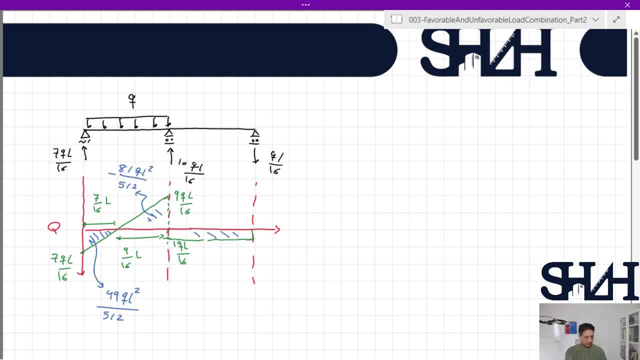 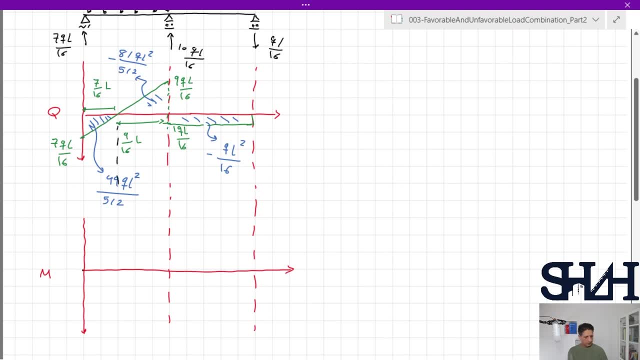 divided by 512, which is negative, and this is q? l square divided by 16.. bending moment will be 0, and then it will go to 49- q, l square divided by 512- and minus 81, 49 be minus 32, and then here we have a line, and 32 divided by 512, 512 divided by 32 will be 16, which. 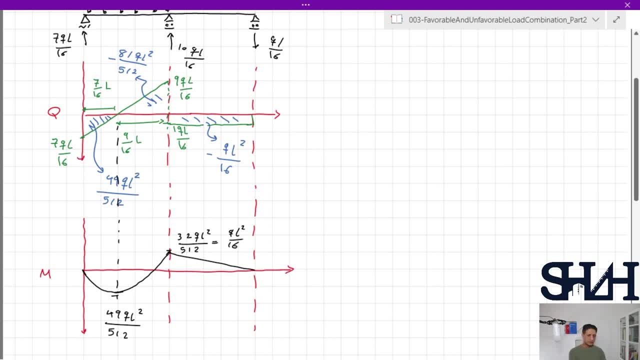 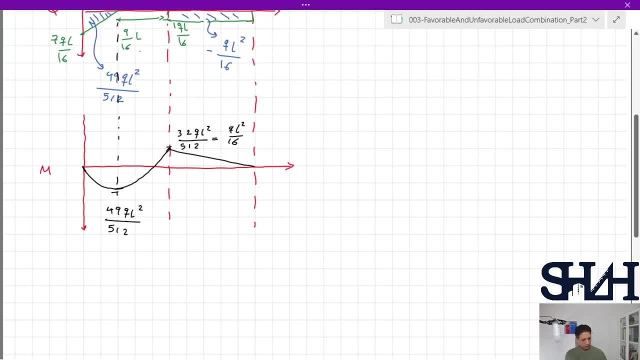 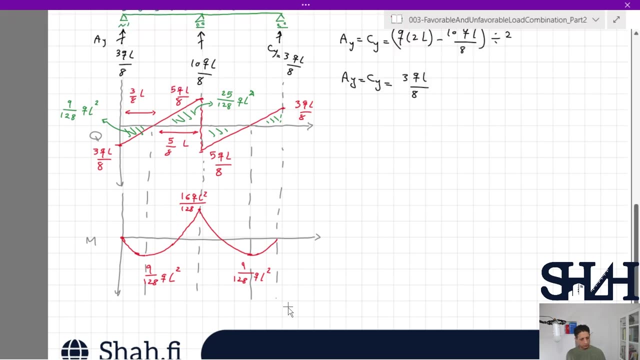 is ql square divided by 16, which is the same value, and it will be 0.. now, if we compare this bending moment diagram of the beam which is under a load only in one span, with the first one, that we calculated for the load to be on both spans and if we want to have the same denominator. 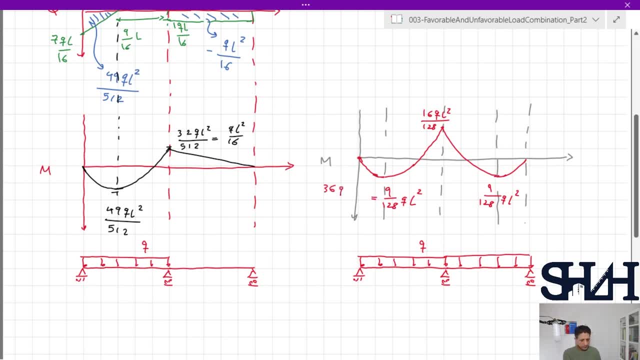 of this, 9 over 128, it will be 36 qls square divided by 512. here we can see that if we have the load only in one span, the maximum bending moment is higher than when we have the maximum when we have the load in two s pants as a. 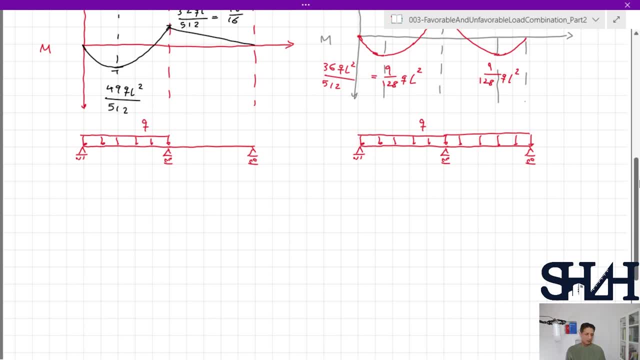 result, if we want to sketch this beam for the most unfavorable bending moment in a span, AB and assuming that the structure is not sensitive to the permanent load, so if most unfavorable case is M between BC, positive bending moment or the maximum bending moment, then it means that we go. 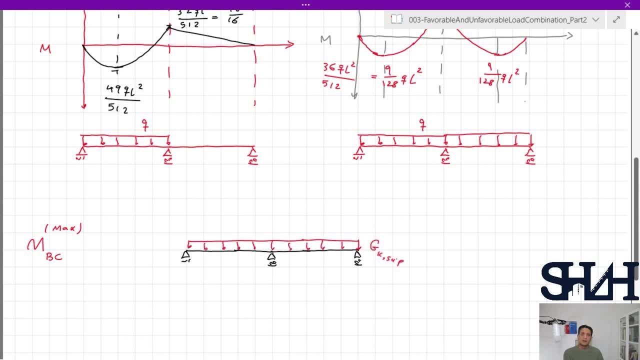 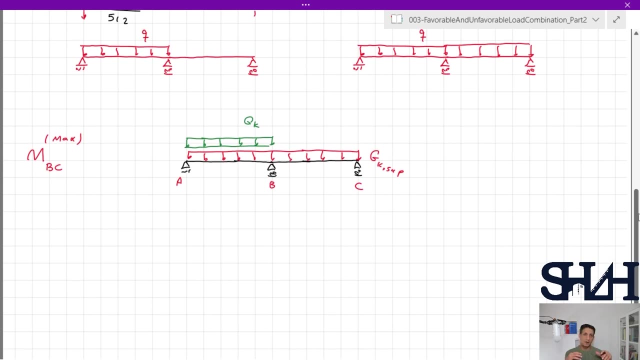 with the GK superior and we apply the live load only on a span AB and you can simply first guess what would be the worst case scenario and then apply the law and if you are interested in the inferior value or most favorable action on MBC, so NBC minimum will be based on GK inferior and Q. 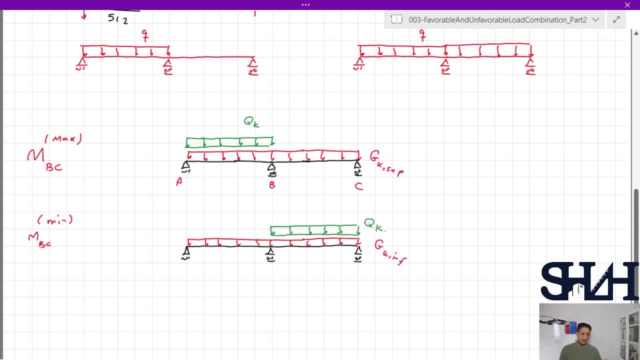 should be applied to the other span for calculation of the maximum bending moment. you can sketch the beam and analyze the beam according to this with the proper partial factor, for example, this can be 1.15 GK superior and this can be 1.5 QK. and here, this can be 1.5 QK and this can be 0.9 GK inferior. 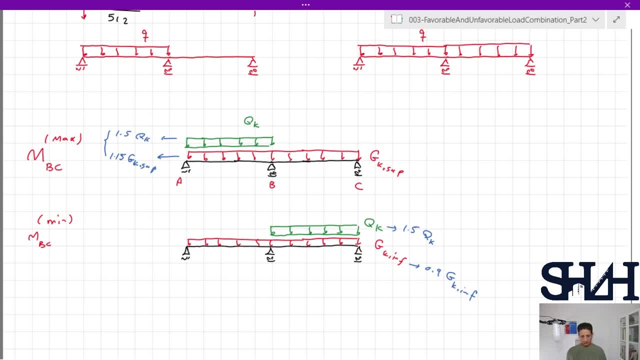 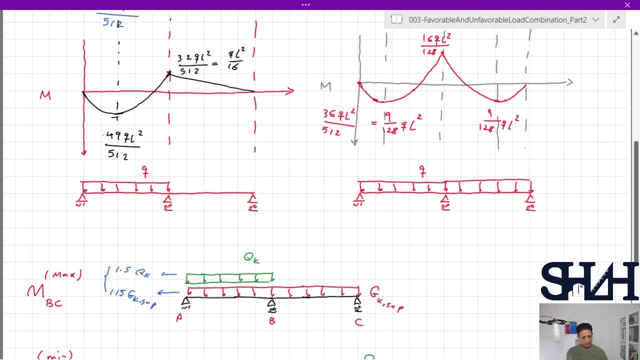 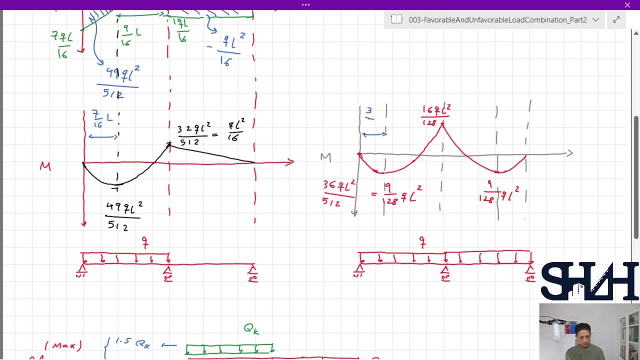 so if you are interested in reasonable approximation, you can take the bending moment from each location, even though they are not exactly in the same position. here we can see that it is in the distance of 7 over 16 L, and this was in the distance of 3 over 8 times L. so 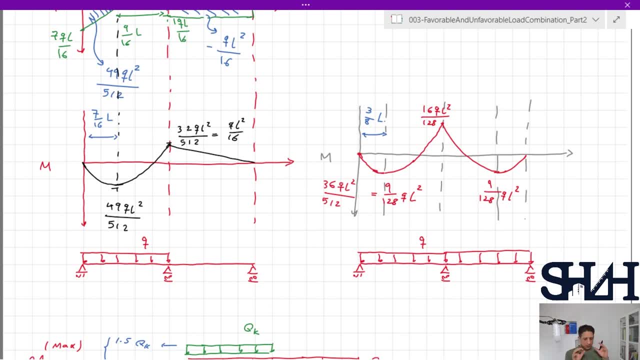 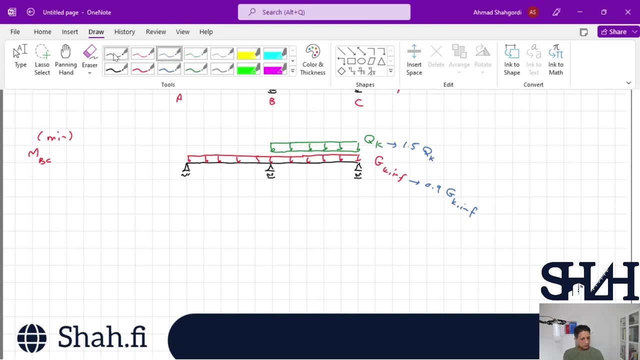 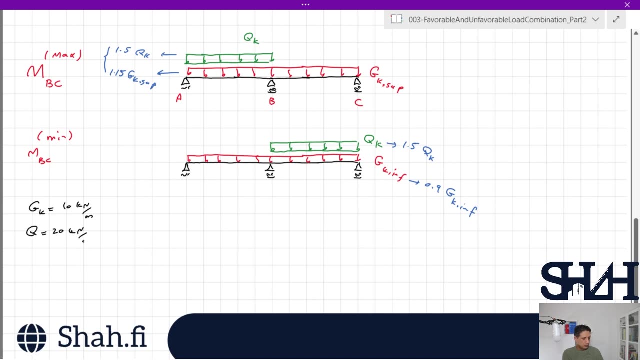 they are not in the same location but it can have a good approximation. let's have some numerical values here. let's assume GK is 10 kilonewton per meter and Q is 20 kilonewton per meter, with the length of, let's say, 6 meters. so for calculation of the most unfavorable action on BC, so it will. 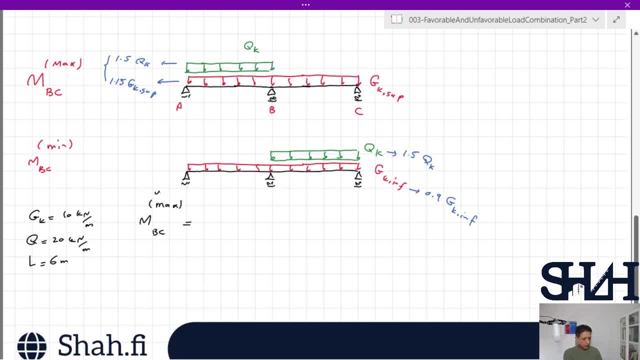 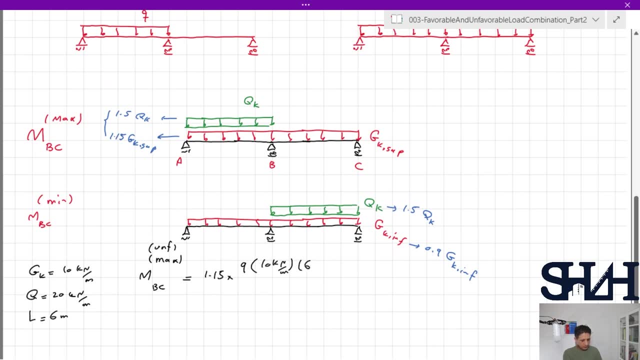 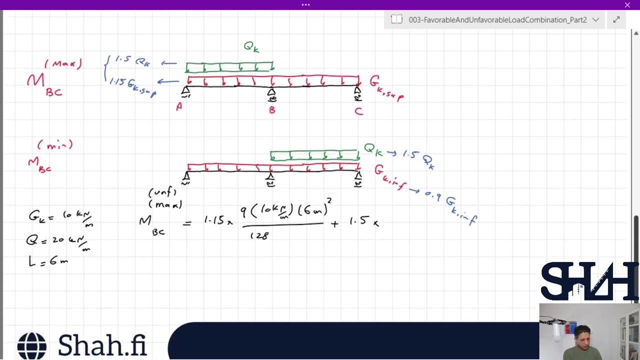 be 1.15 or, most unfavorable, 1.15 times 9 times 10 kilonewton per meter, times 6 meters power by 2, divided by 128 plus 1.5 times. the other one was 49, 49 times 20 kilonewton per meter times. 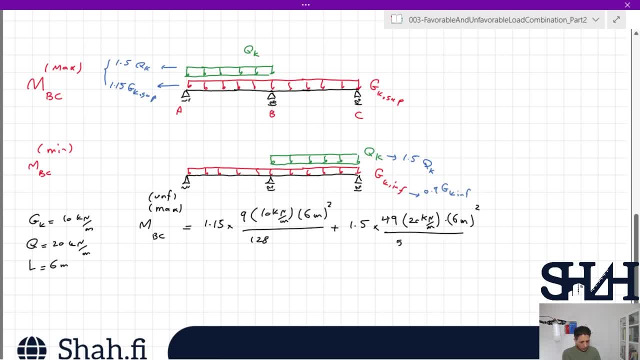 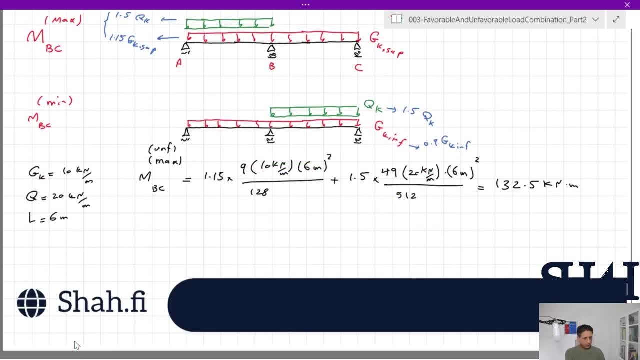 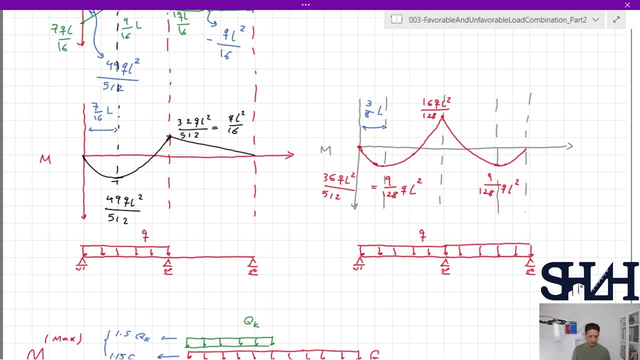 6 meters power by 2 divided by 512, and it will be 132.5 kilonewton meter for the most favorable action. if we come back to here, we can assume this: this beam is symmetrical, so we can assume that we are combining this maximum positive and then this negative value from the live load to be in. 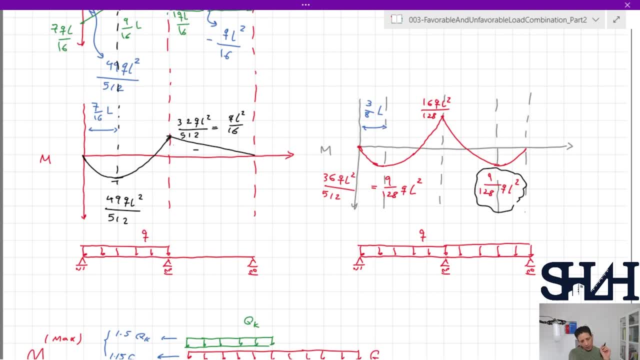 the other span. it's the same here in the support. both are negative and gradually this live load effect is reduced. the bending moment due to live load is reduced, but on the other hand for the span is increased to 9 over 128 QL square. so the maximum might happen somewhere here between the. 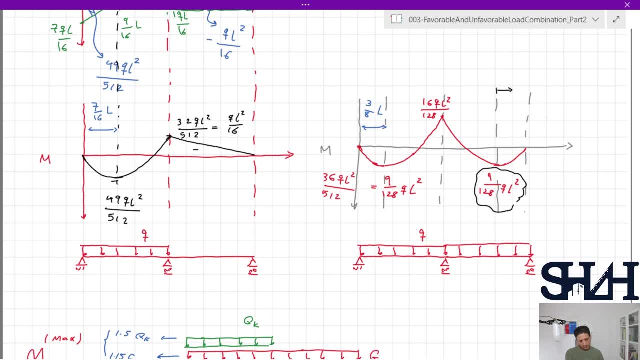 uh, the load, the maximum load, and then the effect of live load. uh, non, 9 over 128 QL square times 0.9 might be reasonable to be assumed, excluding the effect of the live load in the other span, if you are interested in maximum. 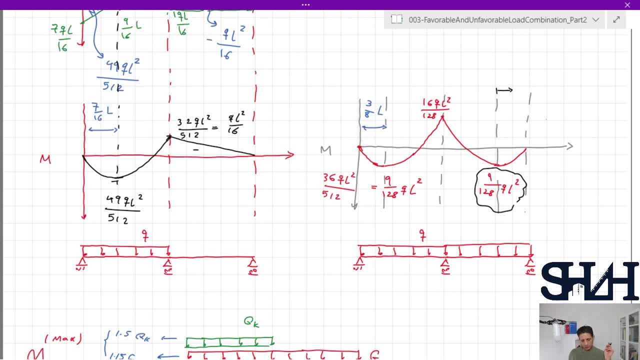 positive bending moment. that is one solution. the other one is just calculating for this point, but perhaps it would be zero or even negative, which might not affect your design, because you have maximum negative in the support. uh, we can try, and in the next video I'm going to solve the same.